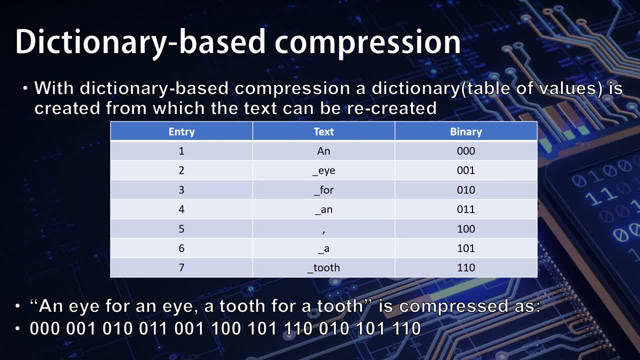 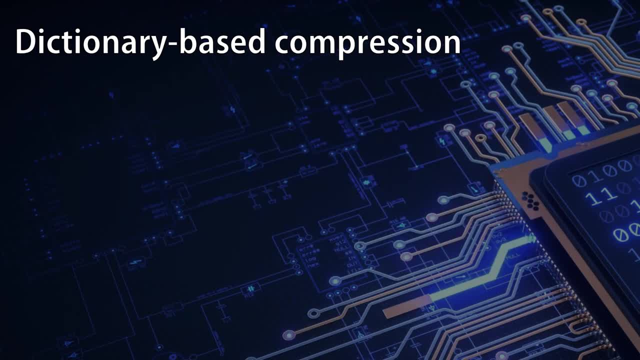 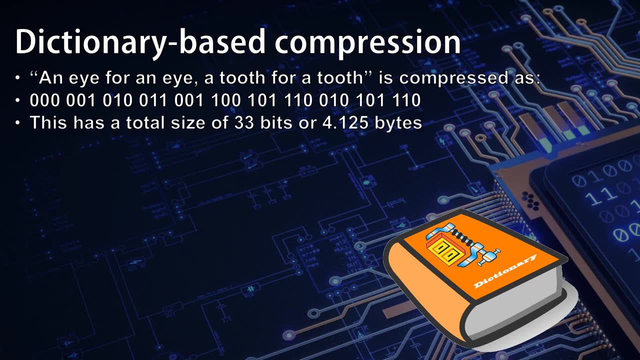 Dictionary Based Compression. Dictionary Based Compression. need to put spaces in there. i just did that so you could see easily which section from the table we were actually using. counting up the bits in our compressed representation of an eye for an eye, a tooth for a tooth, we find that it's got 33 bits, or 4.125 bytes in 8-bit ascii. the phrase has 38. 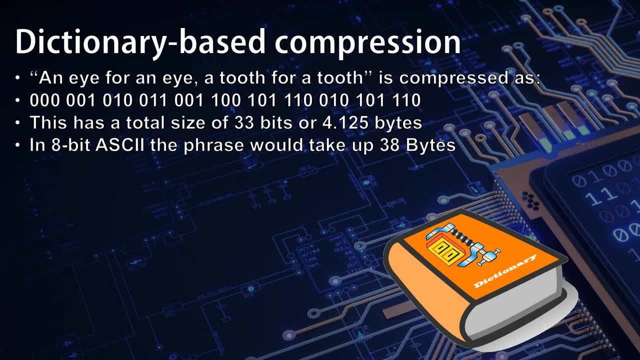 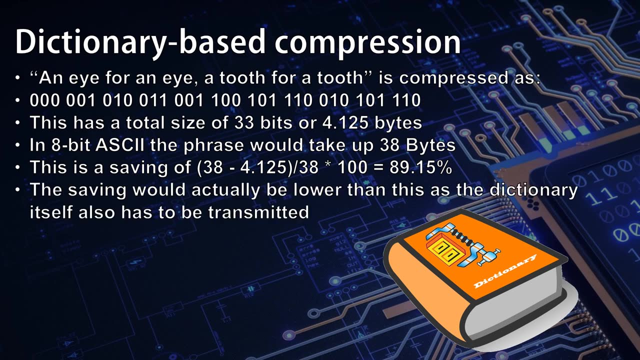 characters, and so would take up 38 bytes. this is a saving of around 89.15 percent. however, this is not the full saving you get with dictionary-based compression. the saving would actually be lower because the dictionary itself also has to be transmitted alongside the message. 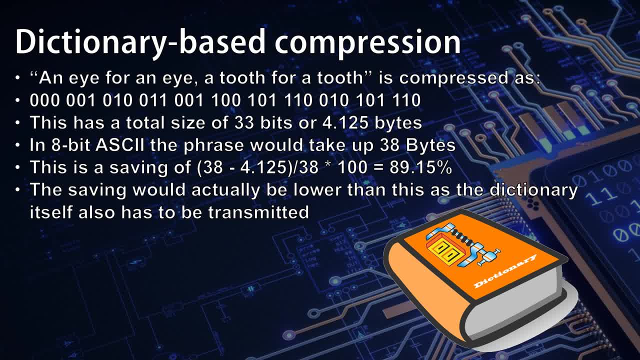 this example shows only a very short phrase being converted to dictionary-based compression. you may be thinking that the size of the dictionary renders it a little bit useless. how the size of the text being transmitted grows in size. the difference between the size of the actual text and the size of the dictionary needed grows a lot, meaning that this is a very effective 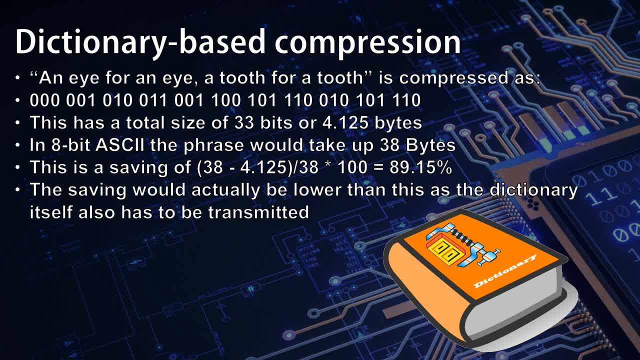 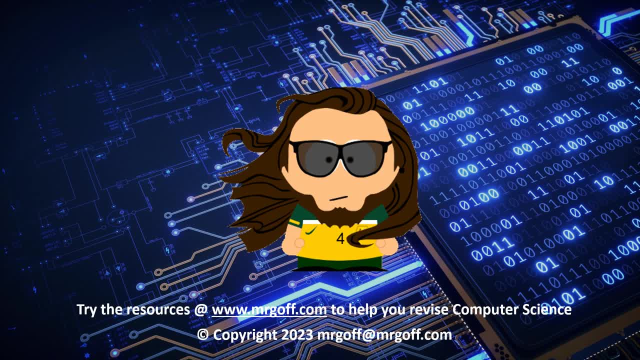 method for compressing large amounts of text. that brings us to the end of this video on dictionary based compression and these videos on the a-level data representation series. join me again soon when i'll be back with new videos for another section of the a-level specification. try the resources.